4,, 5,, 6,, 6,, 7,, 8,, 9,, 10,, 11,, 12.. And if we want equation in x, let's write down y in terms of x. So we can say 1,, 3,, 12,, 3,, 3,, 4,, 5,, 6,, 7,, 8,, 9,, 10,, 12,, 12,, 12.. This is an example. 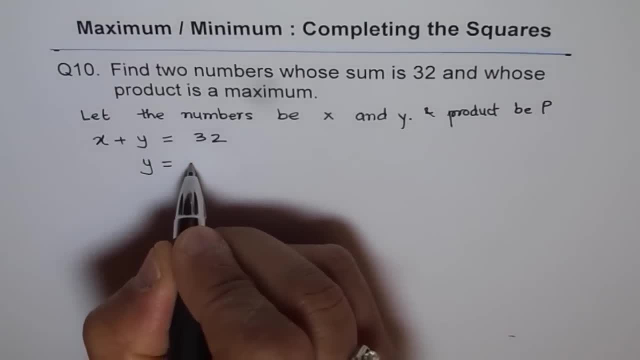 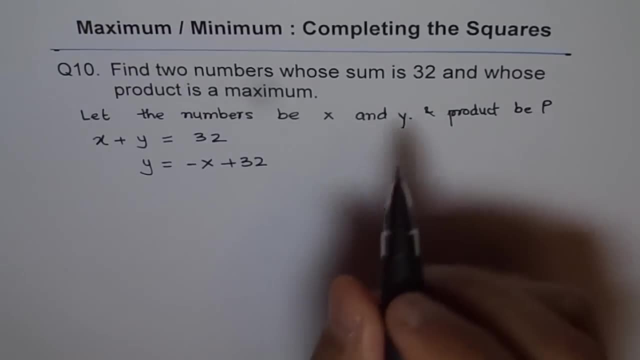 whether we want an equation in x. So now let's say: x plus y equals 32.. And then we need to write: say y is equals to minus x plus 32.. Now let's look into the next statement. Whose product is a? 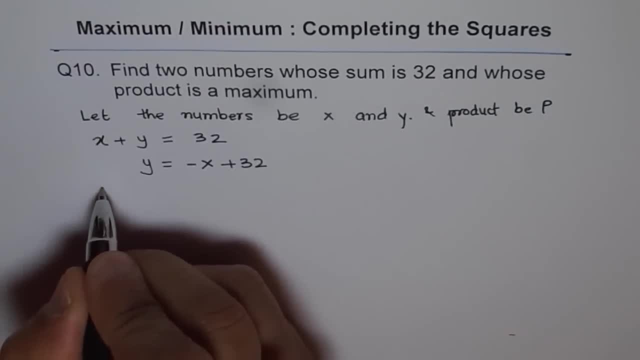 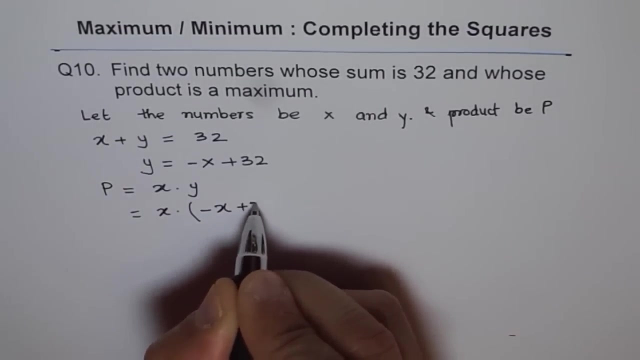 maximum And p is the variable to define product. So what is product? Product is x times y, And now we can write x and y in terms of x X times. let's put this in brackets: minus x, plus 32.. 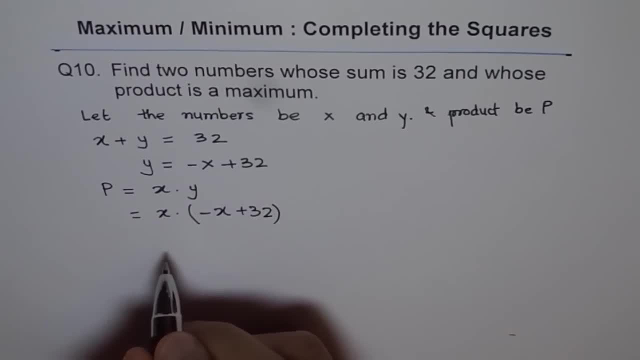 You have to follow all these steps to get really full marks and understand and appreciate the process. So let's open the brackets, So we get minus x squared and x times 32 is plus 32.. X, Correct In comparison, predict the squares. we always factor the coefficient of x square, Here the coefficient 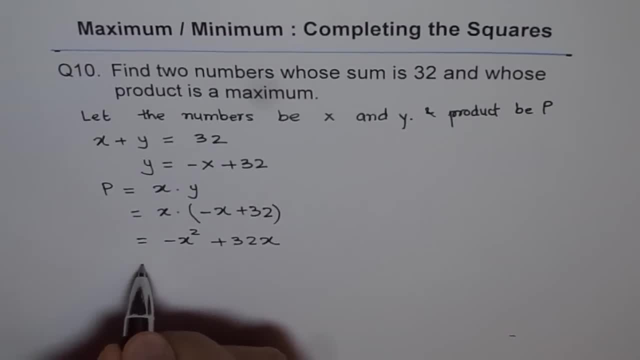 is minus 1.. Do you see that? So we need to factor this. So we get minus outside and I recommend you to put square brackets at this stage. So when you take minus outside, you get x square and this sign changes to minus. See minus times. plus will give you minus right, Minus 32 x. You can verify. 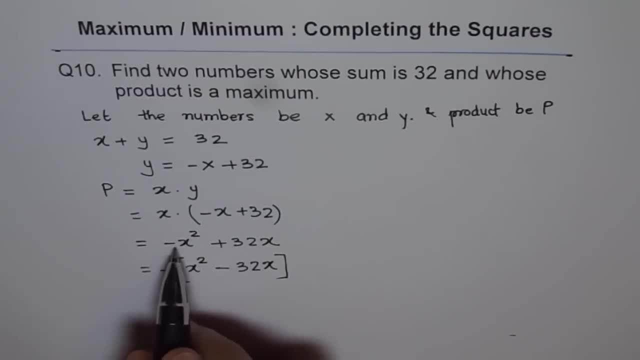 When you expand this, then you get minus x square. that's the first term, and minus times, minus plus 32, right? So that is what you get. Now, what should you do in completing the squares? To complete the squares, we need to half this number, which is 32, half of this is 16.. 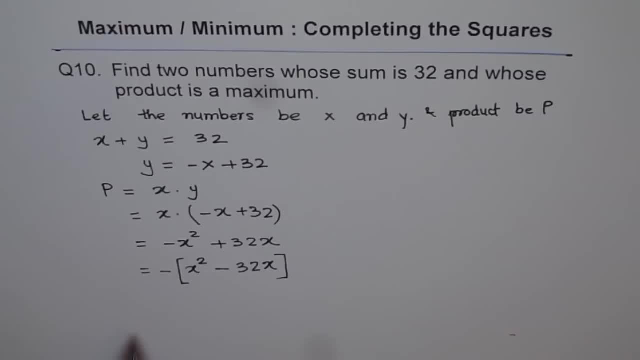 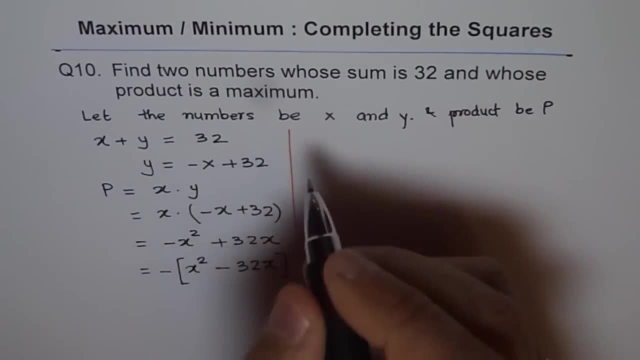 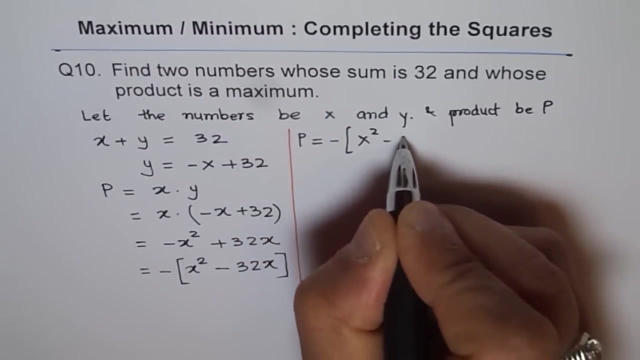 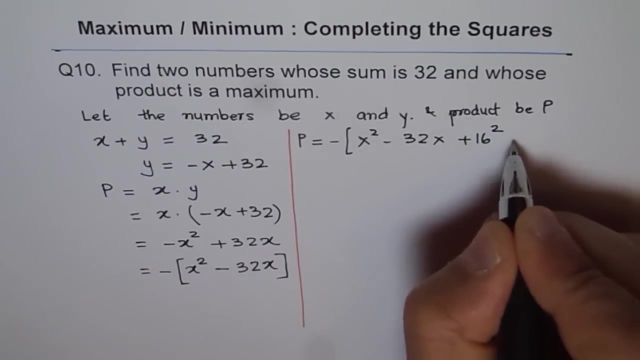 And add and subtract square of that number, correct? Let's do this on the right side. So we have perimeter equals to minus. So we'll x square minus 32, x and half of 32 is 16.. So we'll add and subtract 16 squared. Do you see this? Add and subtract 16 squared. 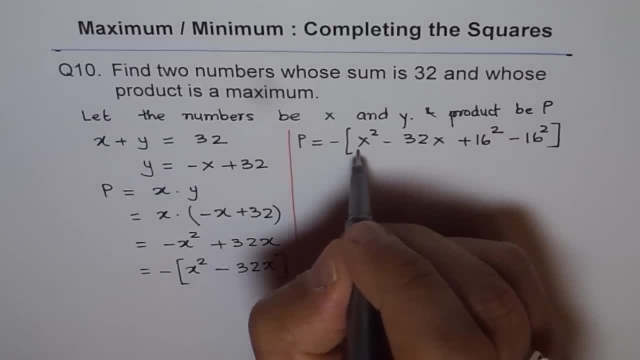 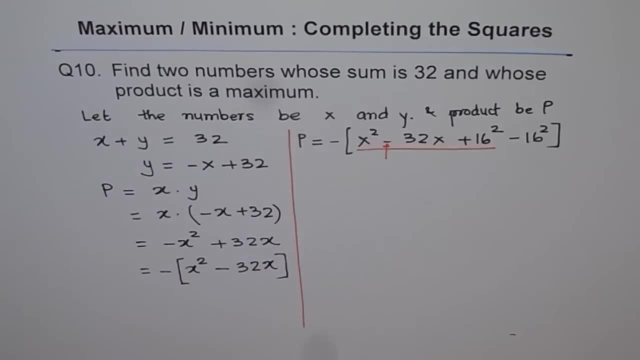 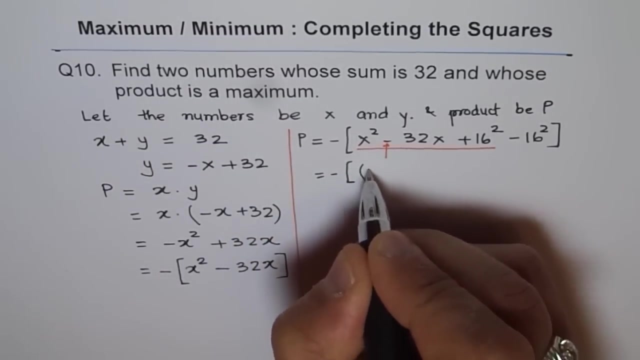 And this will make first three terms as a perfect square, And this perfect square will have minus in it. It is like a minus b whole square, right, So we can write this as minus half. These first three terms become x minus from here. 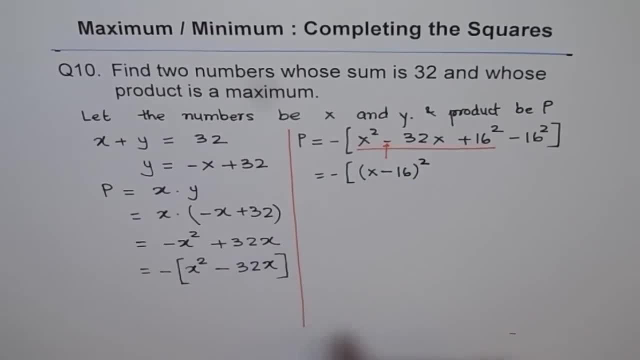 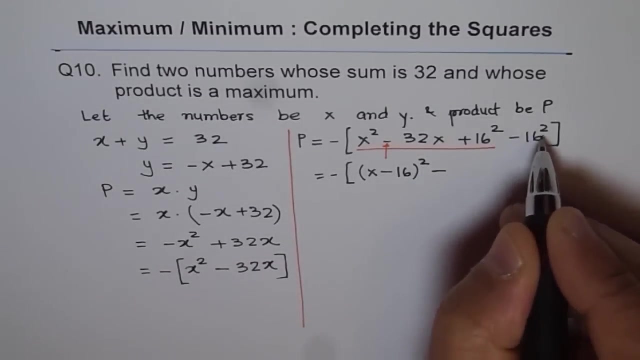 16, from there whole squared. Do you see this? We have taken care of the first three terms: Minus 16, squared Right, Which is 256.. So we can use your calculator and figure this out. So we get minus 16 squared. 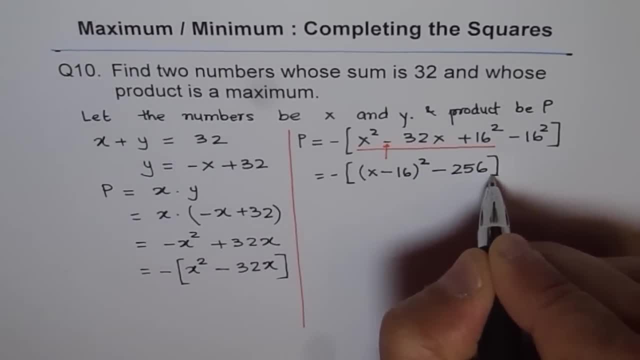 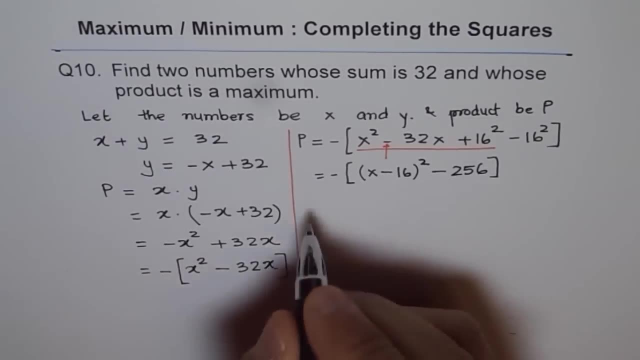 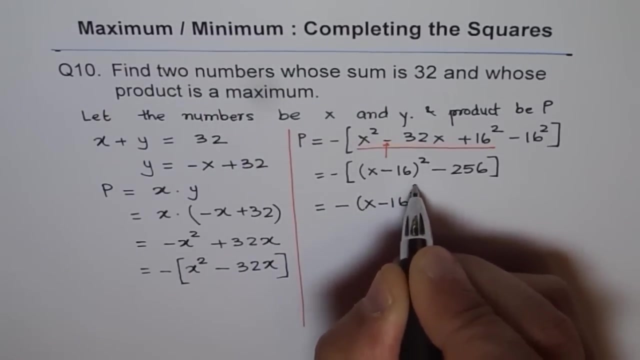 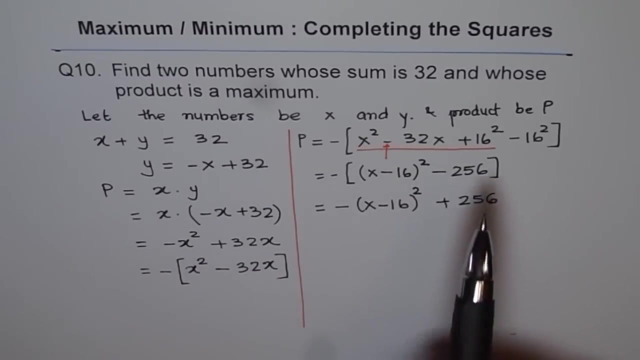 which is 256.. And now, at this stage, we have already done the completing the squares. We should now open the bracket and simplify. So when we open the bracket, we get minus of x, minus 16 whole square plus 256, right Now to get the maximum. this is the vertex of our parabola: To get the maximum. 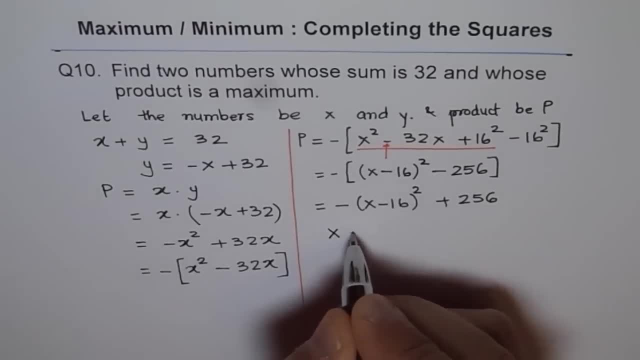 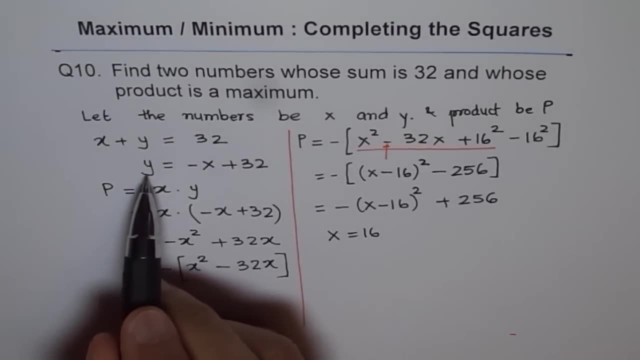 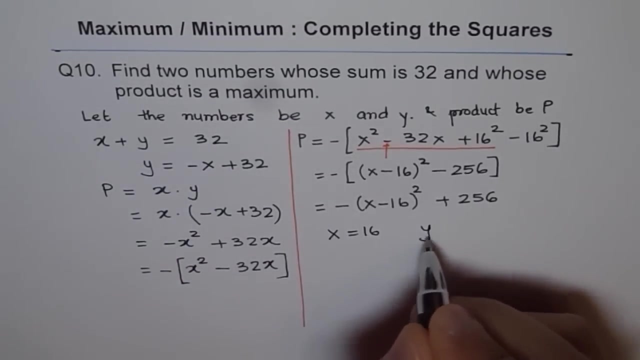 x should be equals to 16, right? So x equals to 16, to get the maximum correct. And if x is 16, then what is y? y will be minus x plus 32, correct? If x is 16, then y is equals to minus. 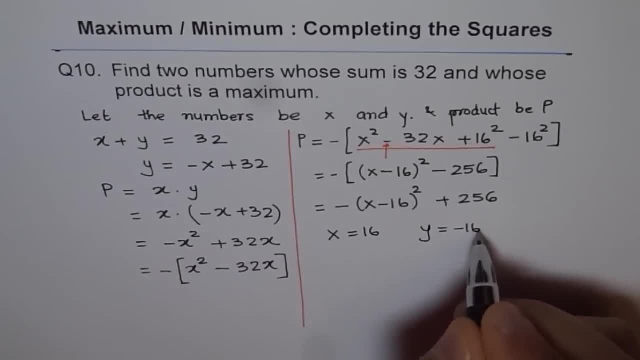 x plus 32.. That means minus of 16 plus 32, right, Which in this case is also 16, right? So in this case, the two numbers which we have got are 16 and 16.. Okay, And their maximum product is 256, right. That is the maximum And maximum product is. 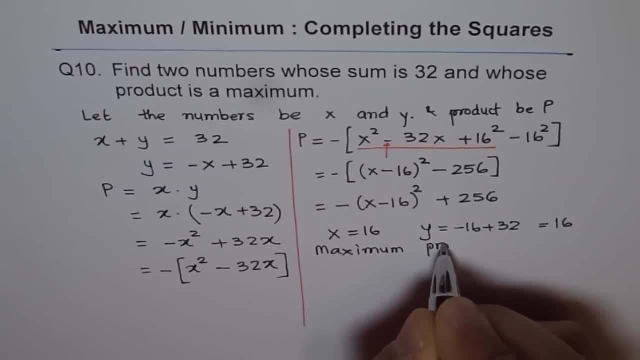 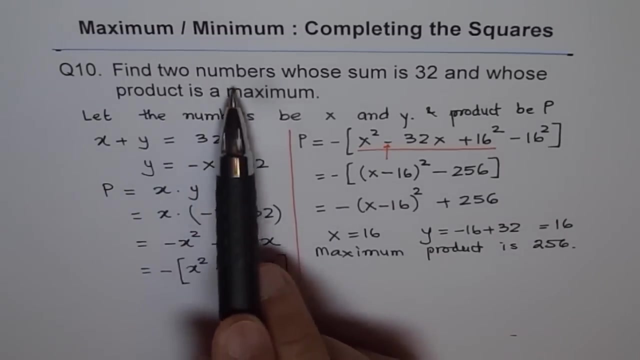 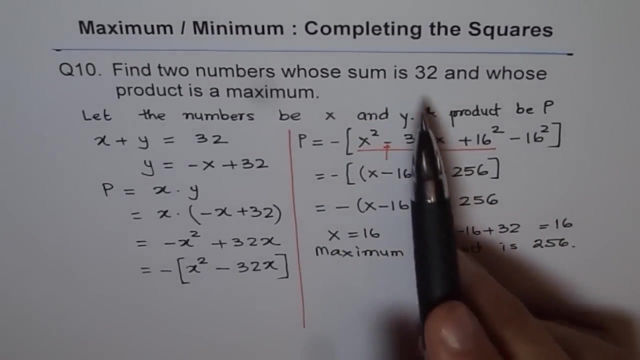 is 155, correct. So that is what you get using this method. right Now. the thing is that find two numbers, So we get two numbers. if we are explicitly finding two different numbers, and let us say the two numbers are integers, In that case the closest number to success.